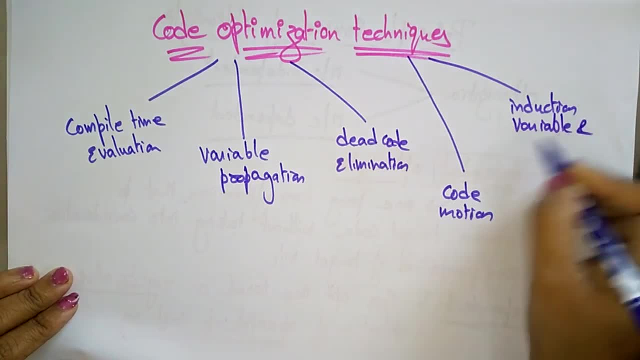 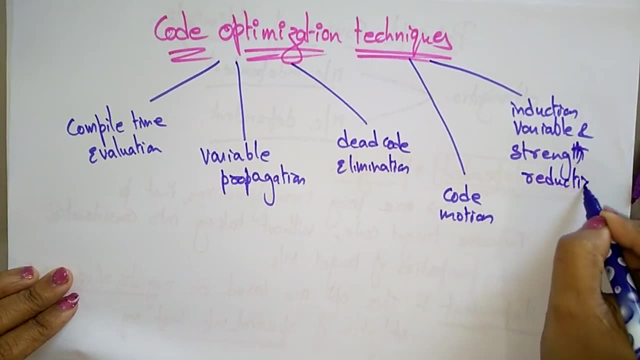 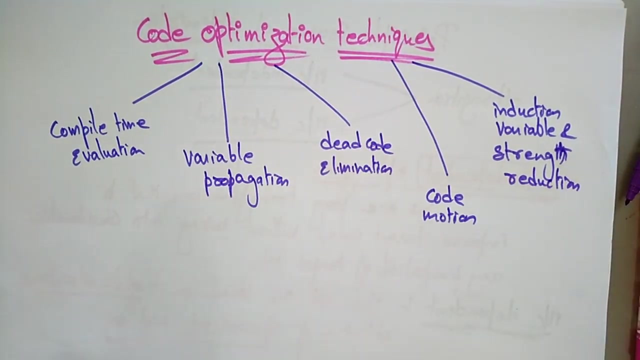 Induction variable and strength reduction. Induction variable and strength reduction. So these are the different, the five techniques of the code optimizing. If you want to optimize the code by taking the front end with the help of the intermediate code, whatever you are taking the source code, that intermediate code is converted. 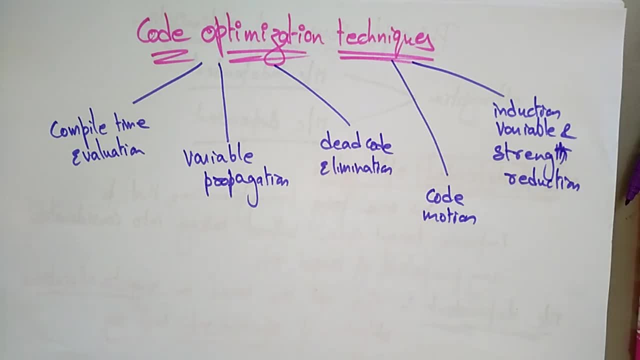 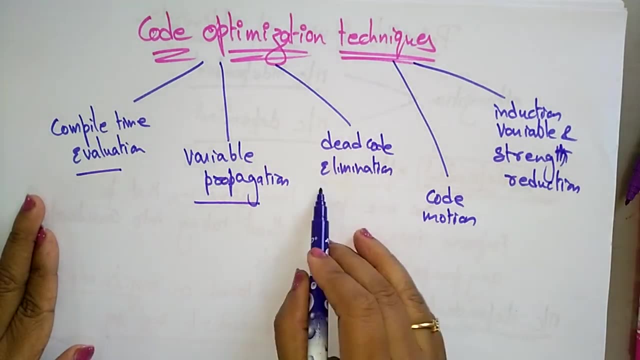 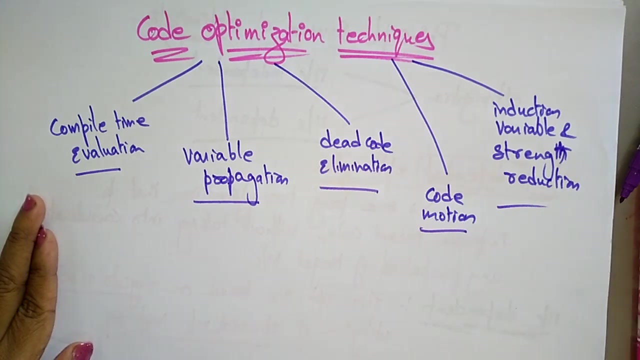 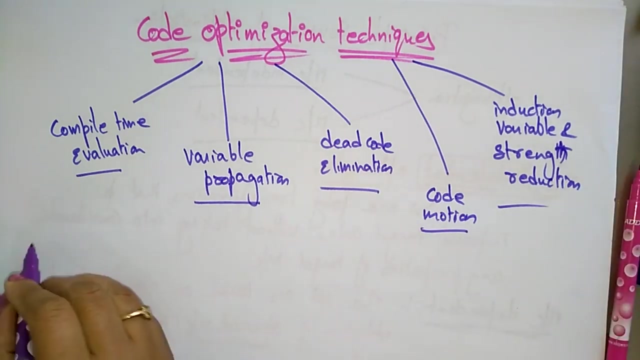 into the code generation. You have to transform the source code into the code generation. You have to transform to the code generation. The code optimization can follow the compile time evaluation: variable propagation, dead code elimination, code motion induction variable and strength reduction. Okay, So now let's see one by one. So what is this compile time evaluation? first, Let's take 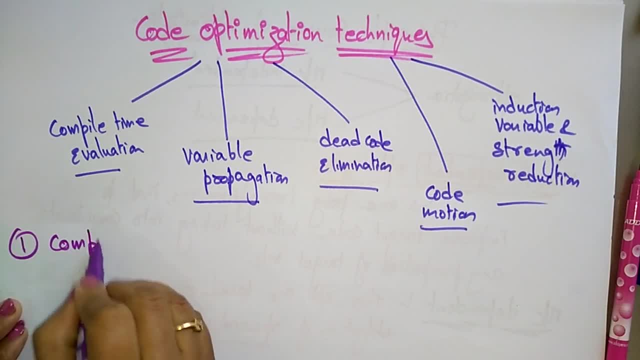 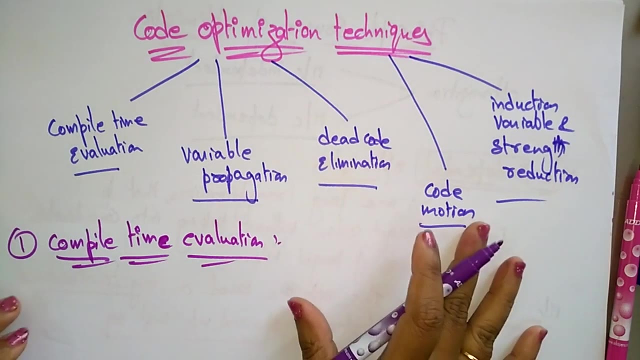 each technique one by one. The first technique is compile time evaluation. Okay, So by seeing this word, what do you understand? What is this compile time evaluation? So let me take an example to explain this compile time evaluation. Let's take one equation. 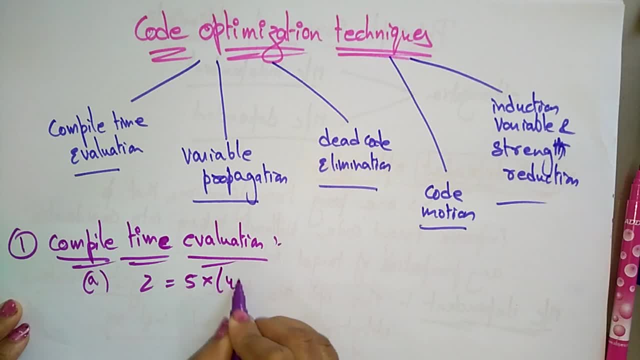 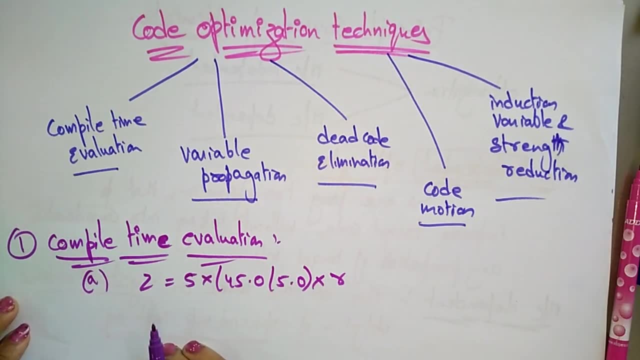 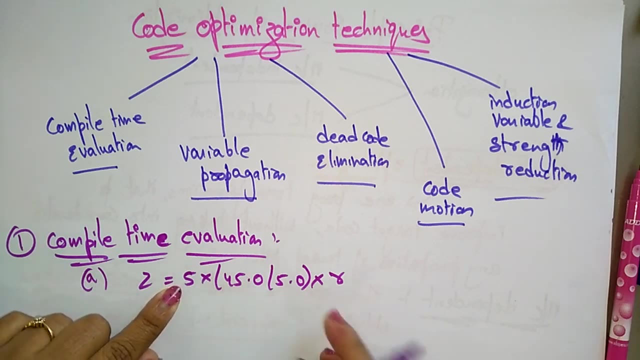 Z is equal to 5 into 45.0 by 5.0. into- let's take R. Okay, So it is going to perform 5 into 45.0 by 5.0.. into r at compile time. So this equation is going to be execute at compile time. 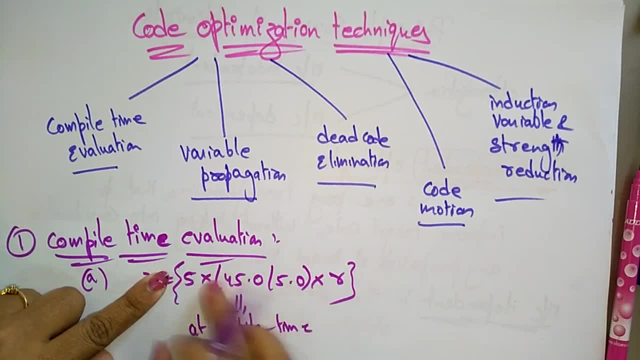 So it does not bother about what is the z here, it is just going to execute whatever this evaluation is there. So let us take another expression. suppose x is equal to 5.7 and y is equal to x by 3.6.. So now the compile time, what it is going to be evaluate. It directly evaluates. 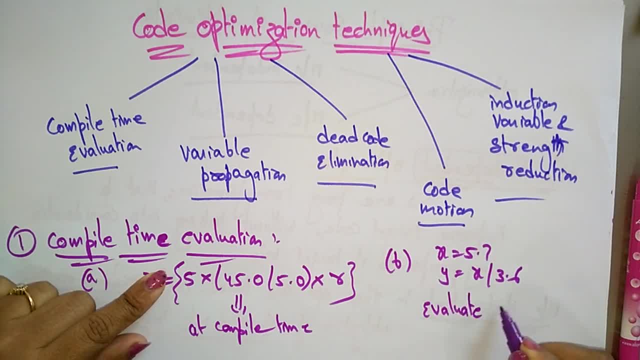 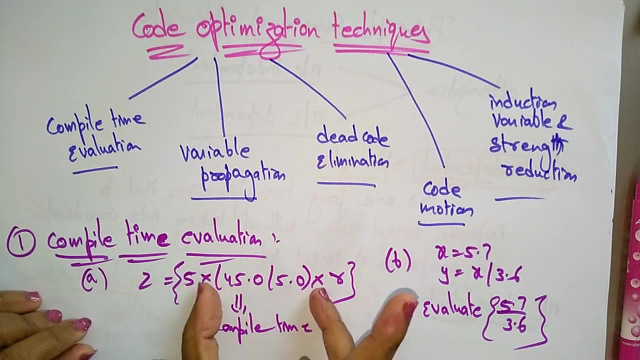 it. the compile time evaluates 5.7 by 3.6 directly. ok, It is directly. substitute the value here and evaluate this expression at compile time. So this is the compile time evaluation. So whatever that we want to be executed, that will be executed. If any variables, if you want to insert any values. 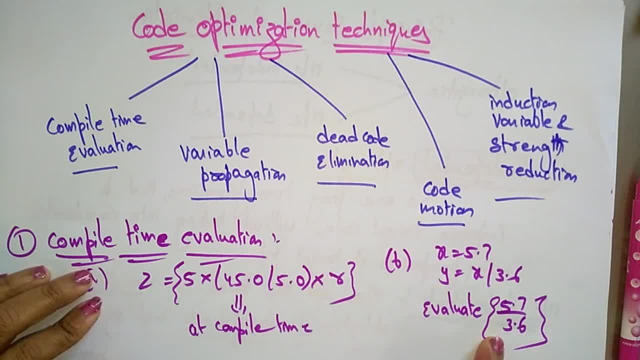 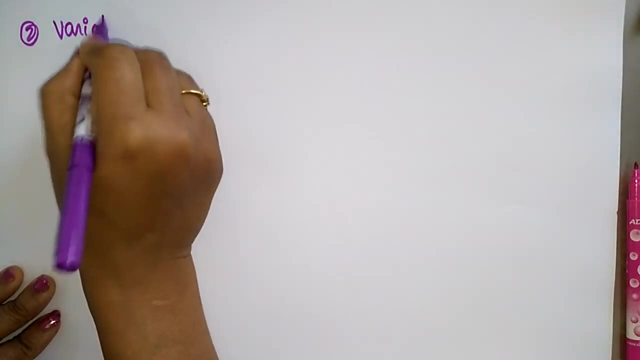 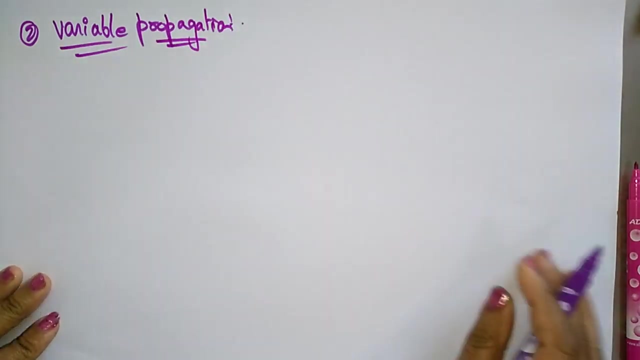 for that variable it insert and execute, ok. So this is the compile time evaluation. Directly, it is evaluating. So next is the variable propagation. So what do you mean by variable propagation? The second one is variable propagation. So let me take an example to explain. 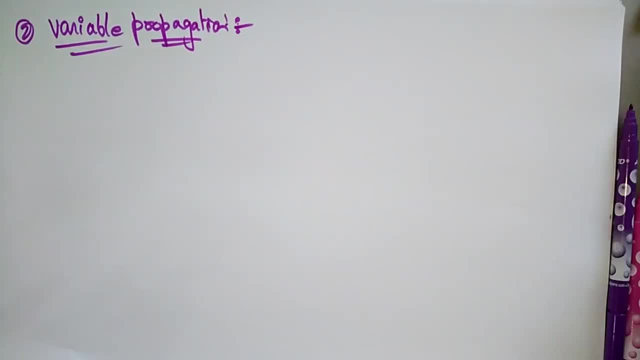 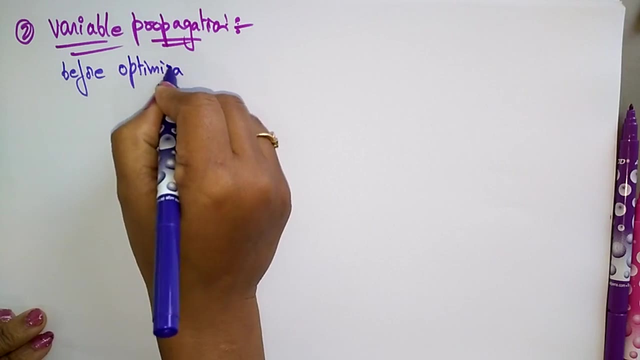 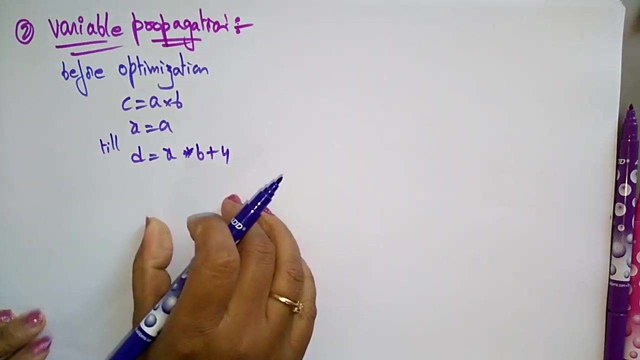 about this variable propagation. So before optimization, let us take the code. Before optimization, let me take a code: c is equal to a into b and x is equal to a and you have to till: d is equal to x into b plus 4.. So this is before optimization. Let us see the code after. 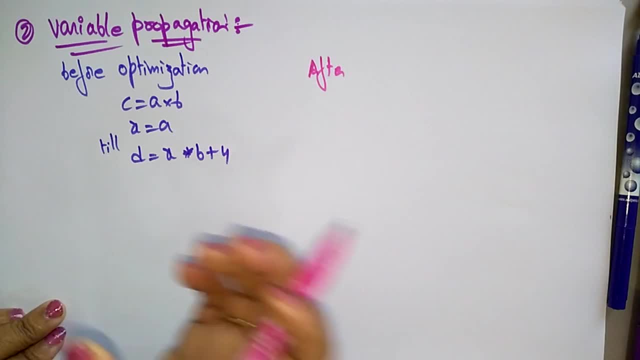 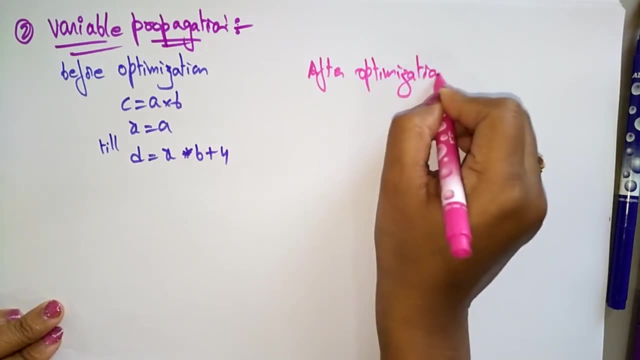 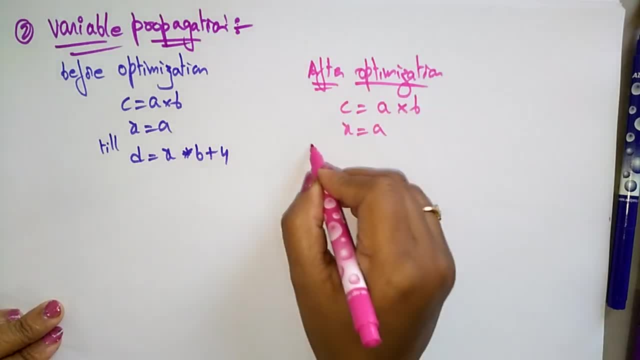 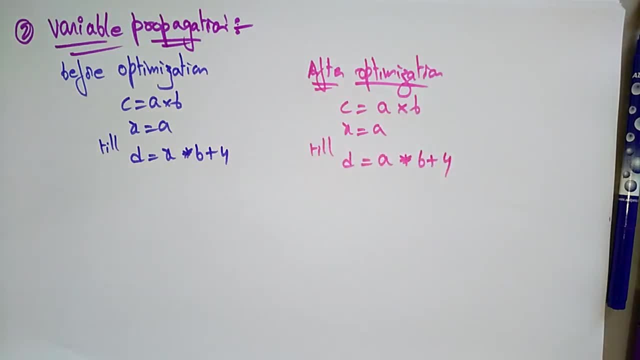 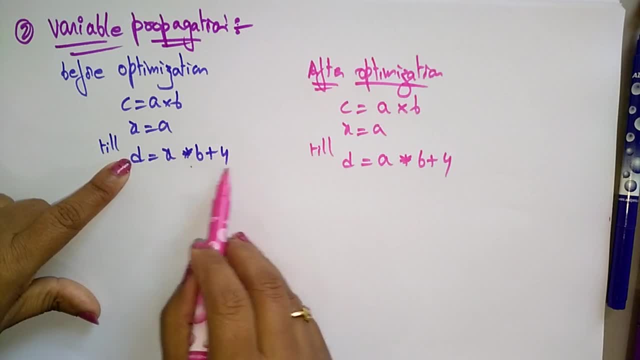 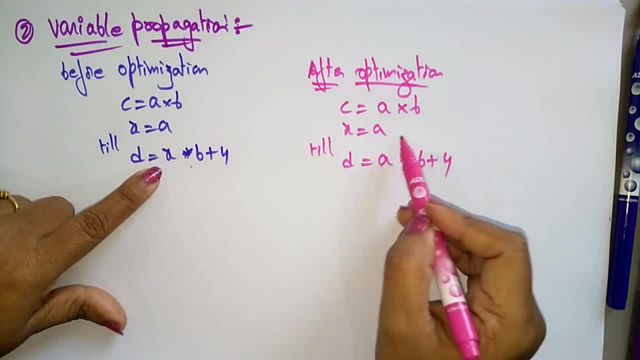 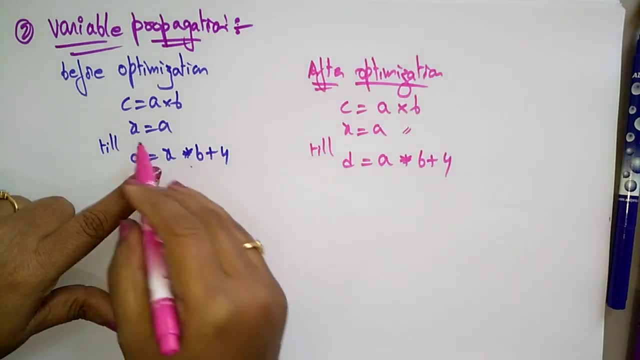 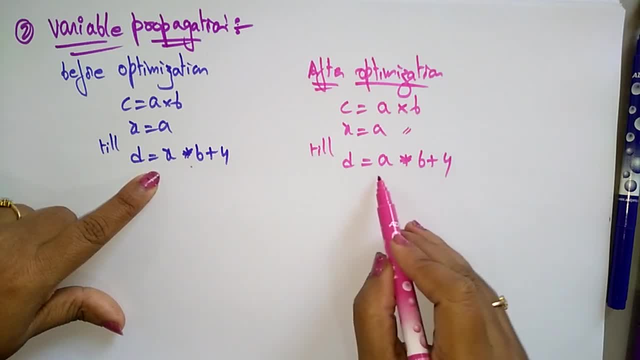 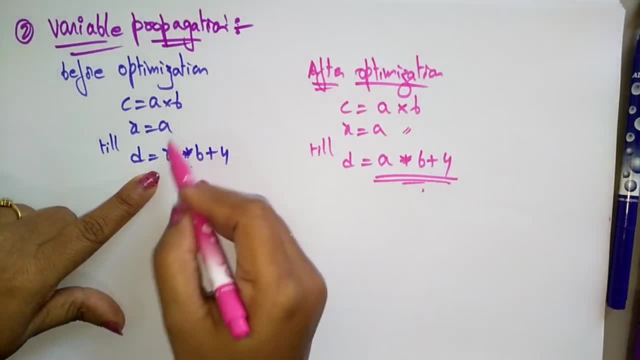 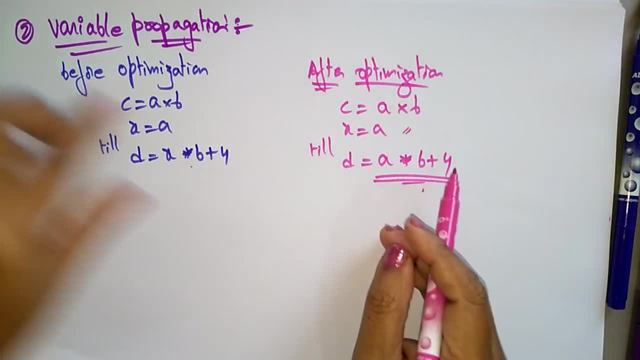 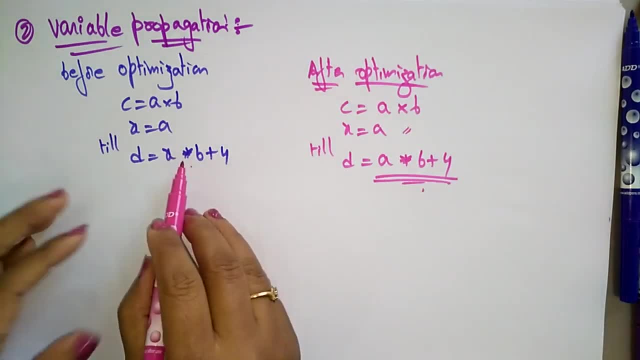 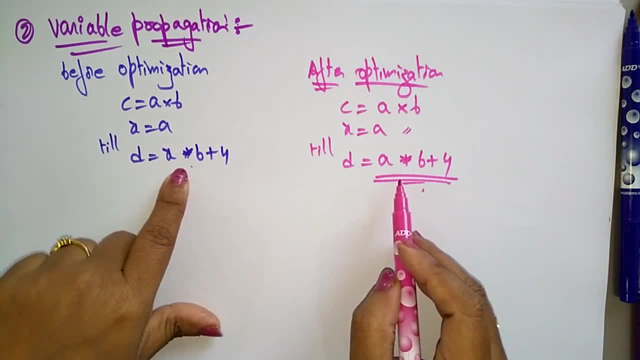 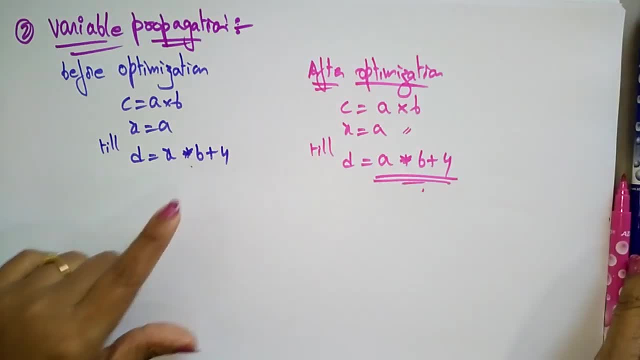 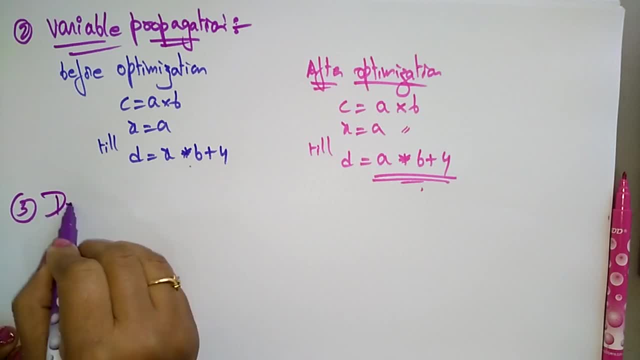 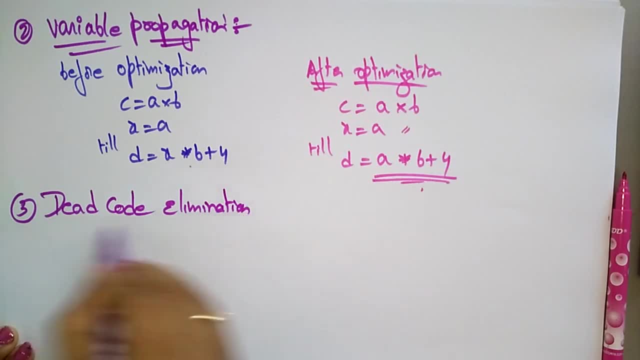 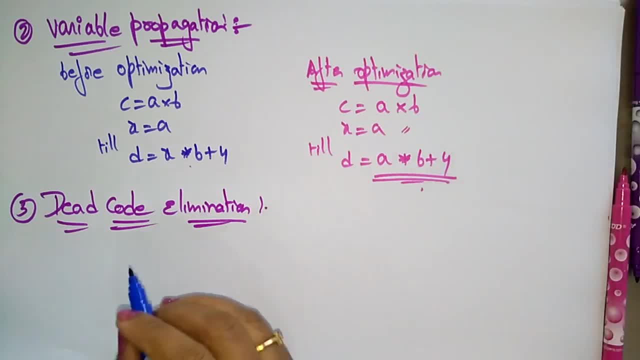 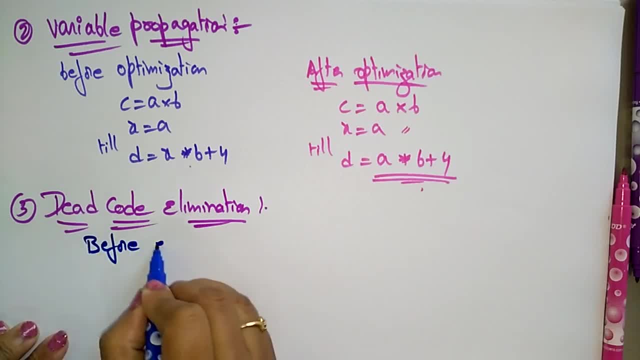 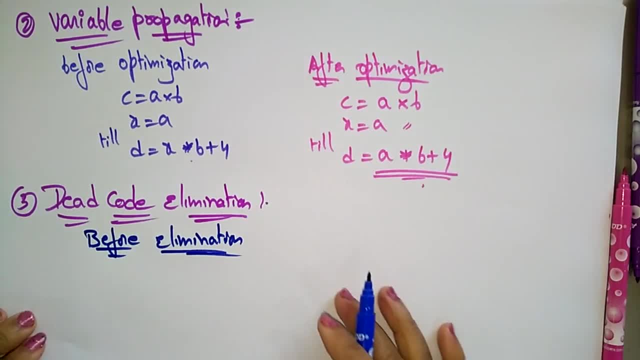 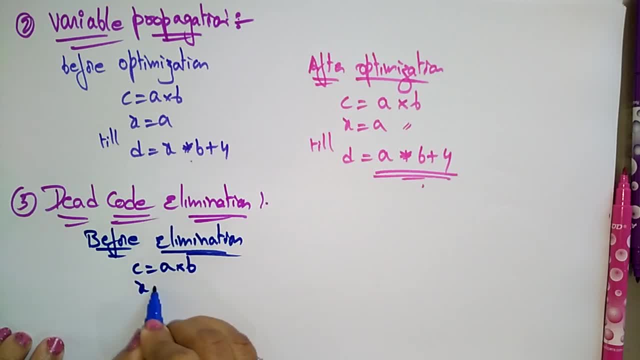 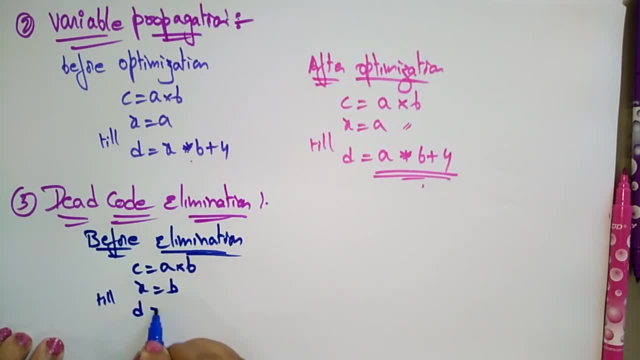 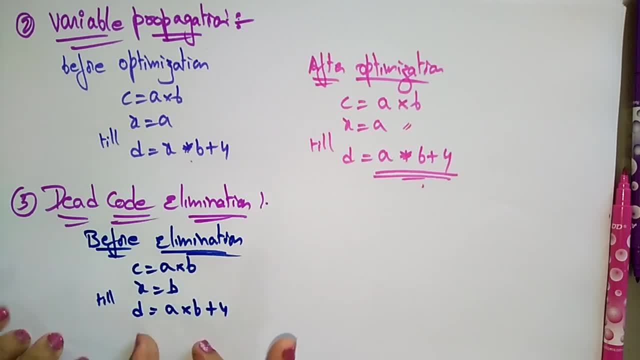 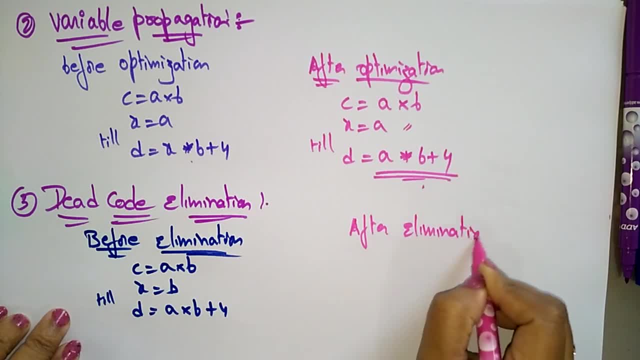 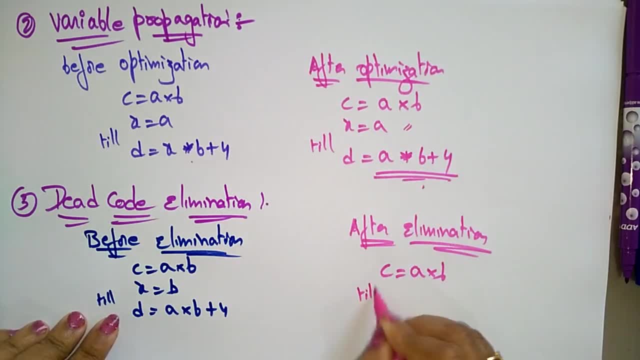 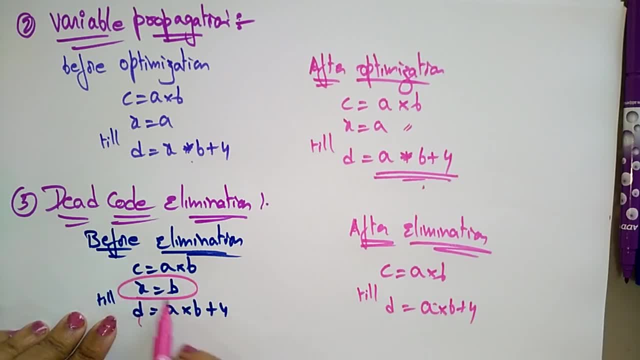 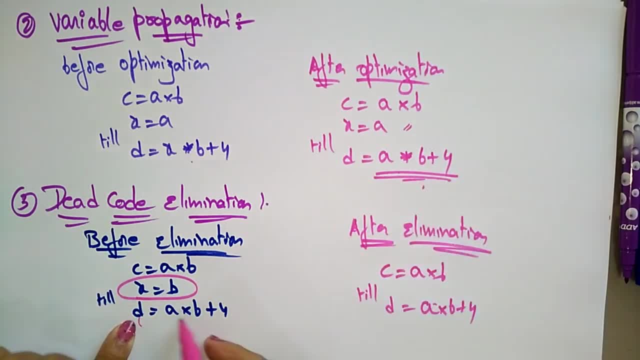 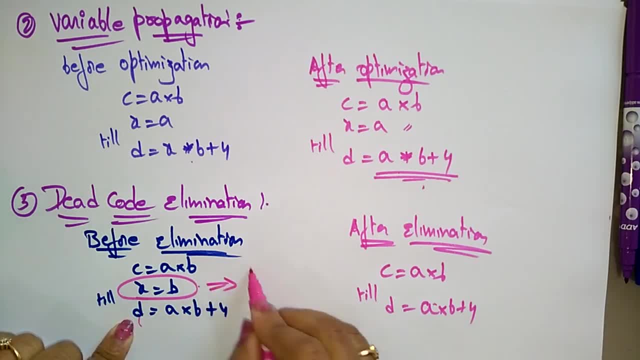 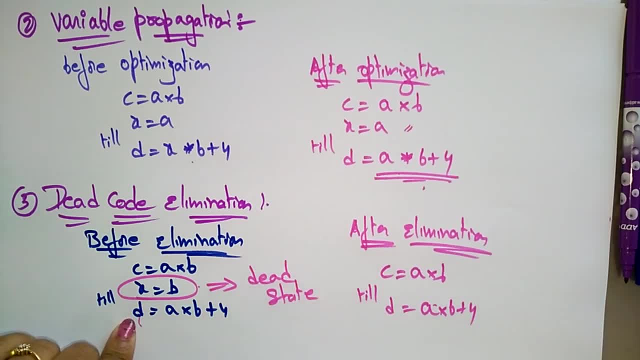 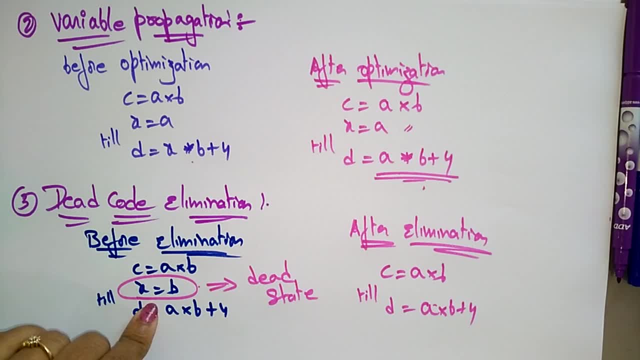 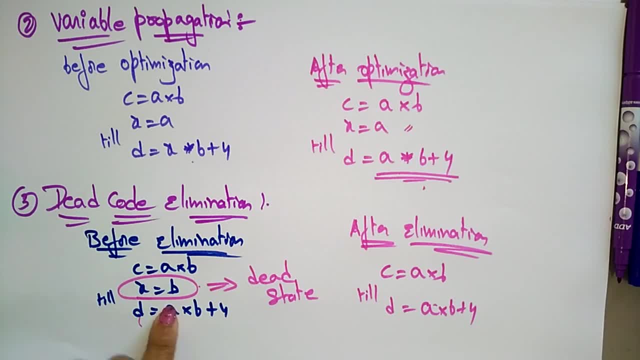 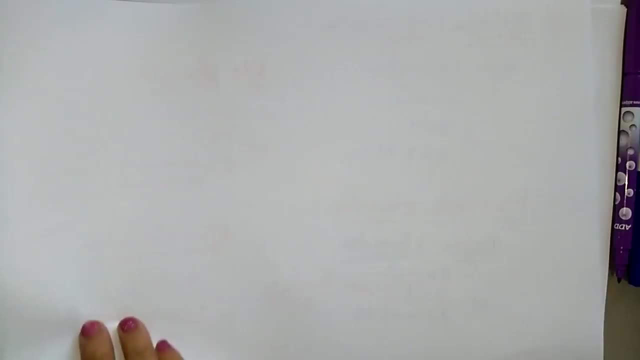 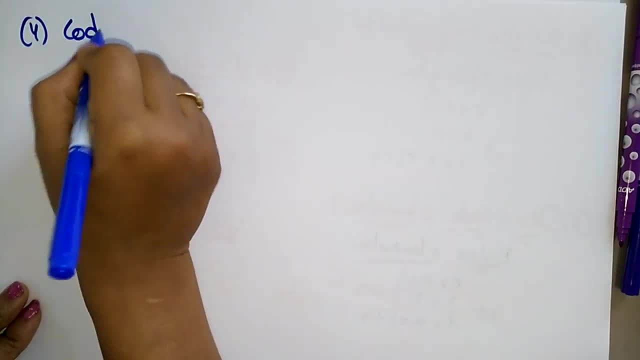 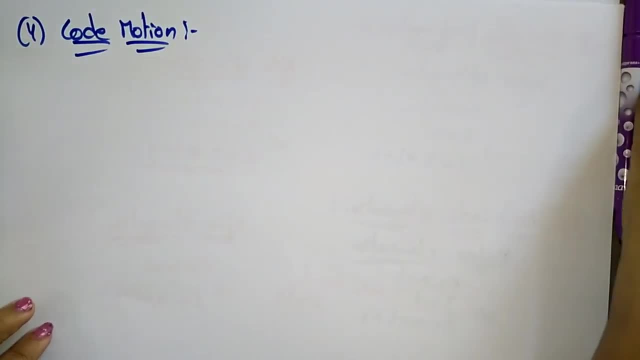 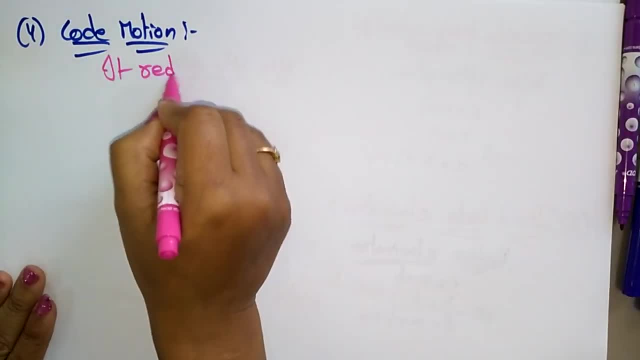 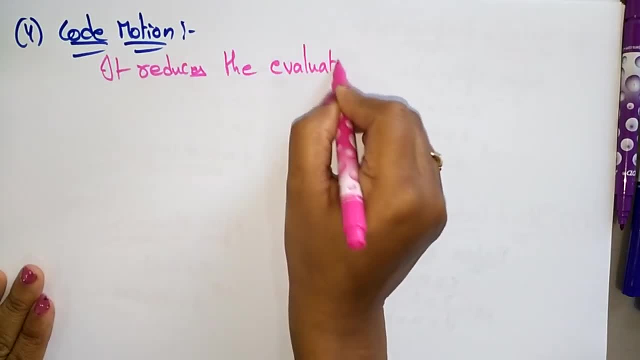 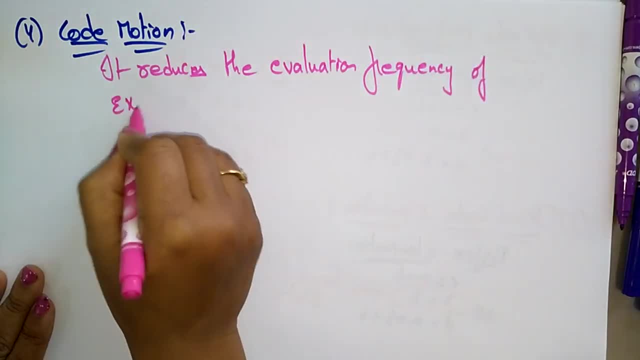 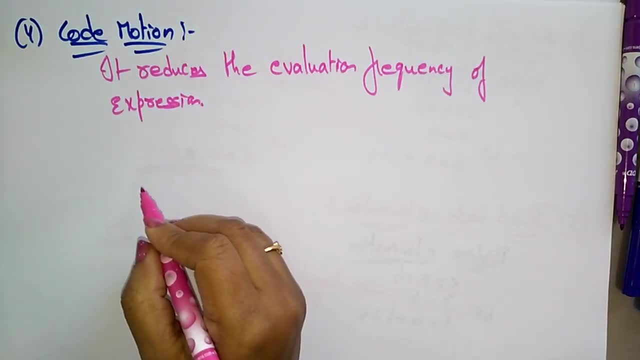 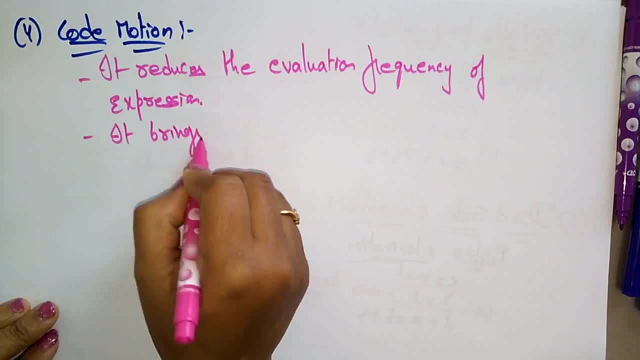 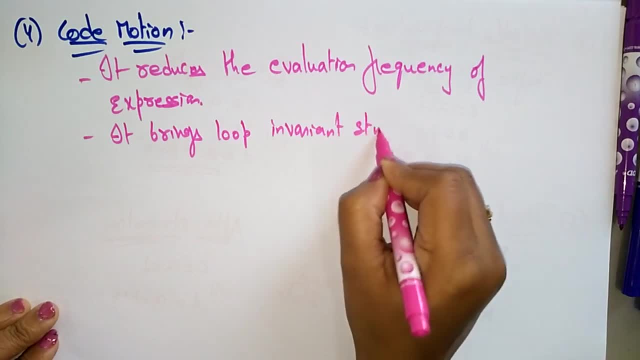 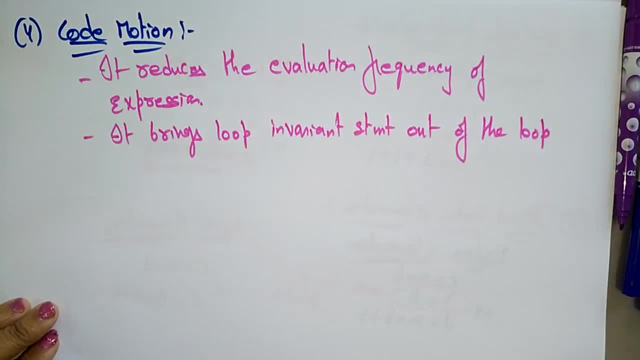 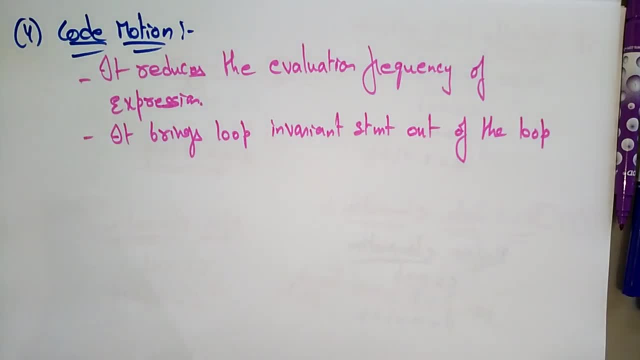 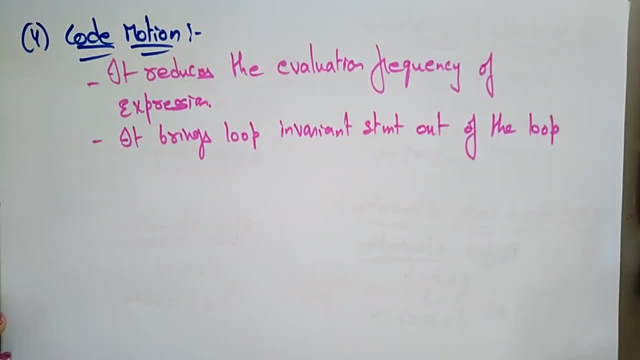 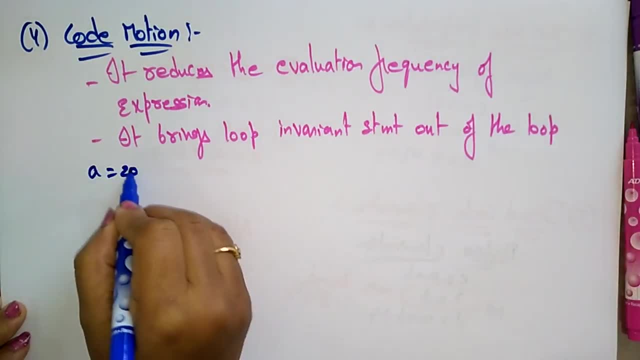 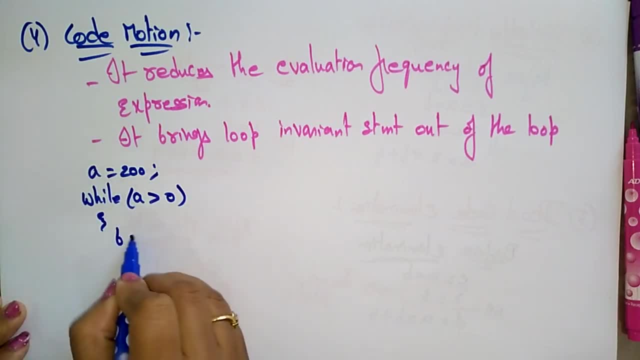 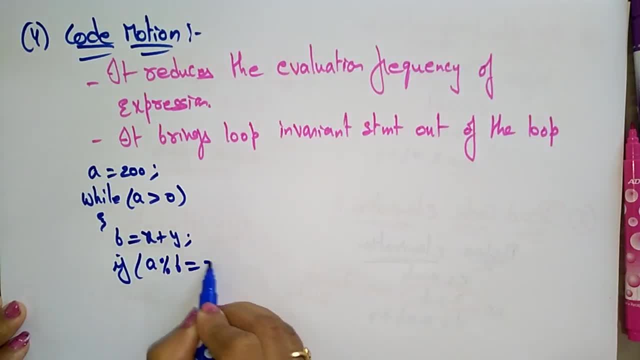 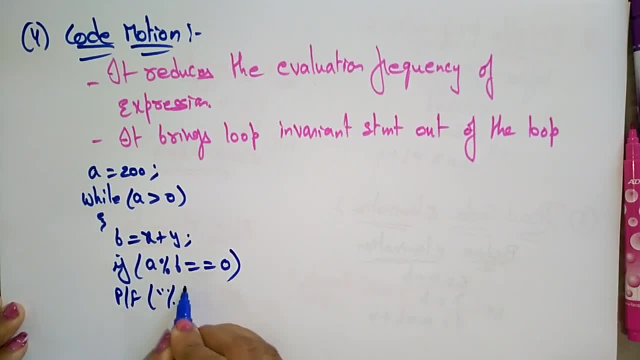 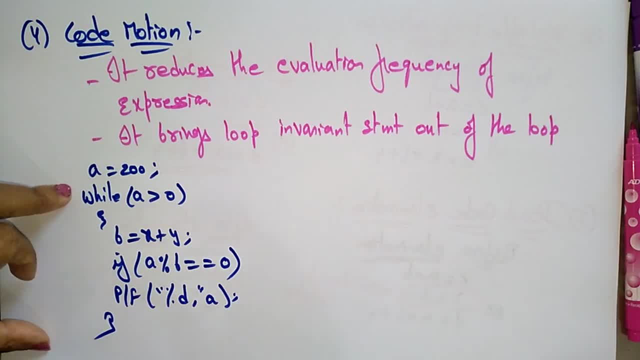 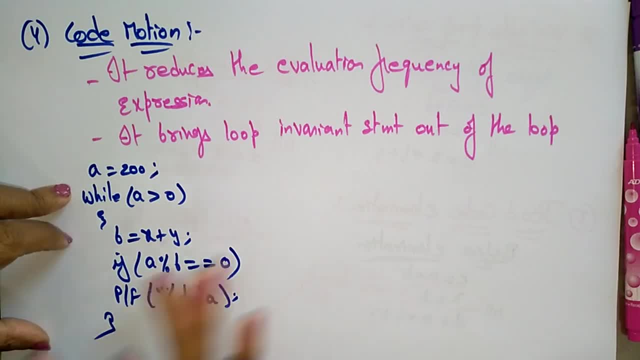 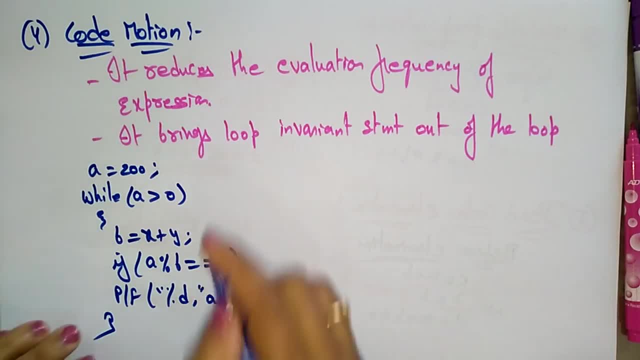 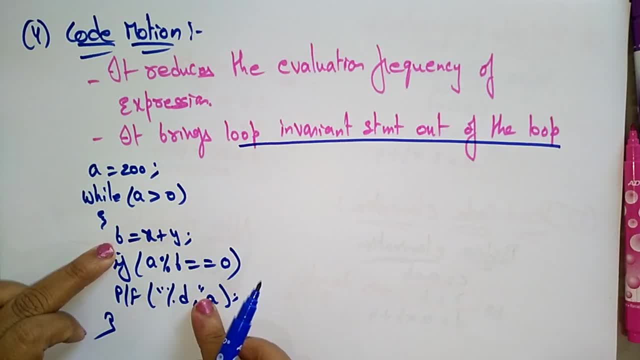 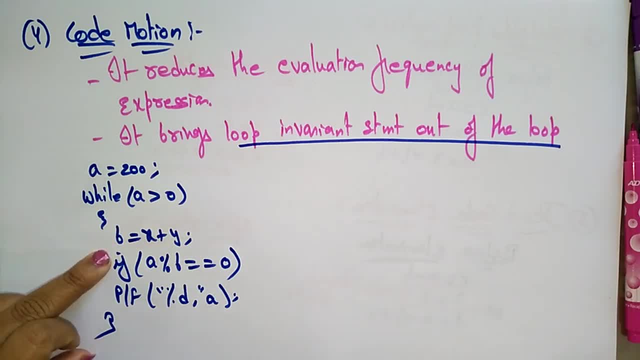 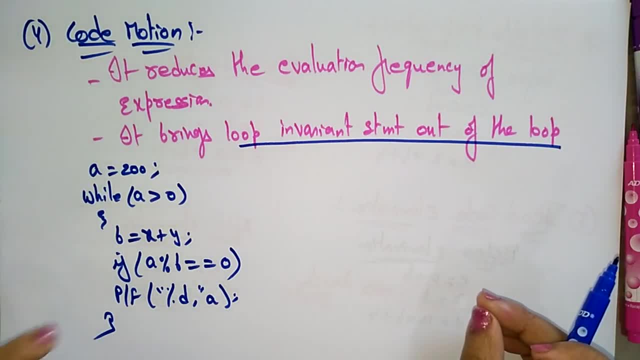 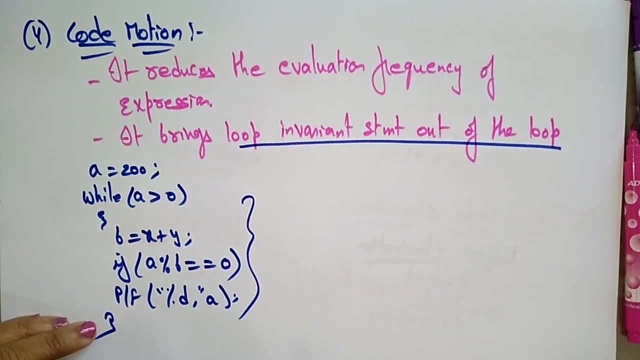 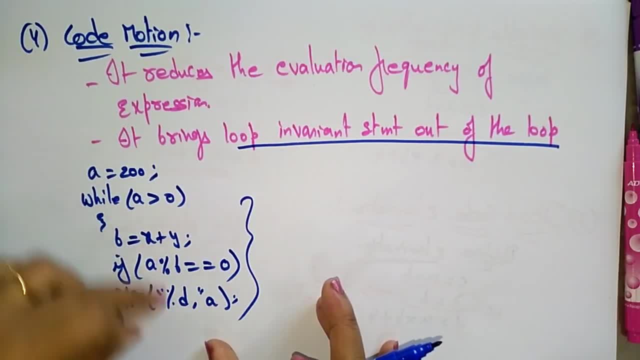 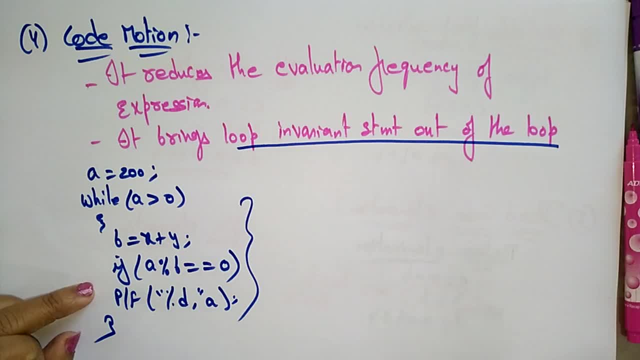 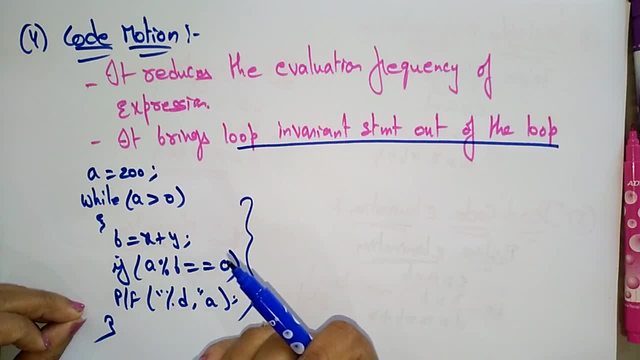 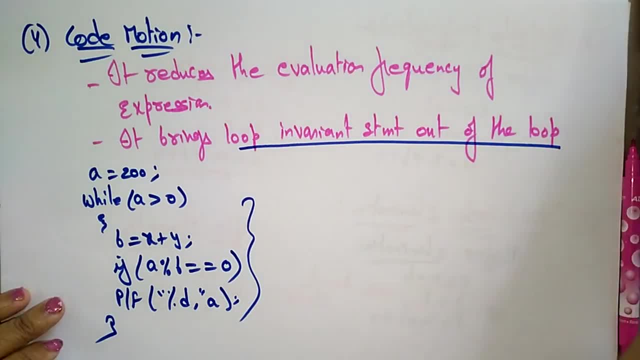 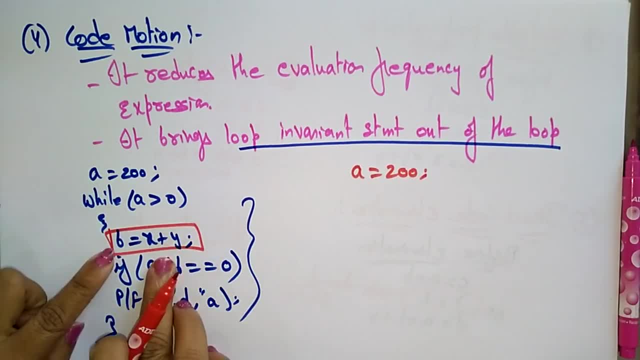 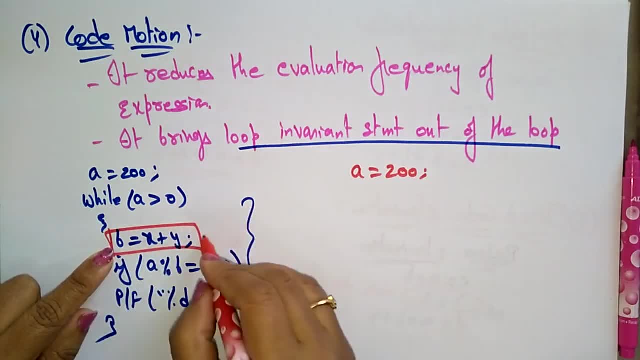 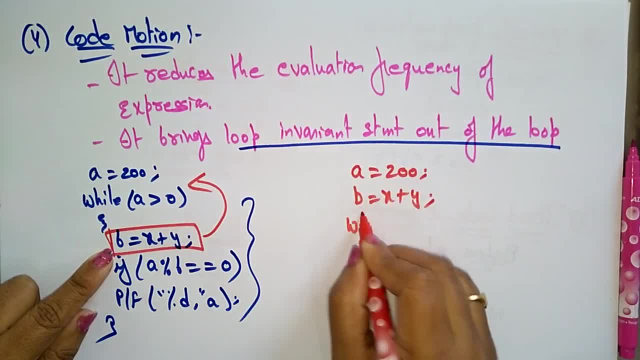 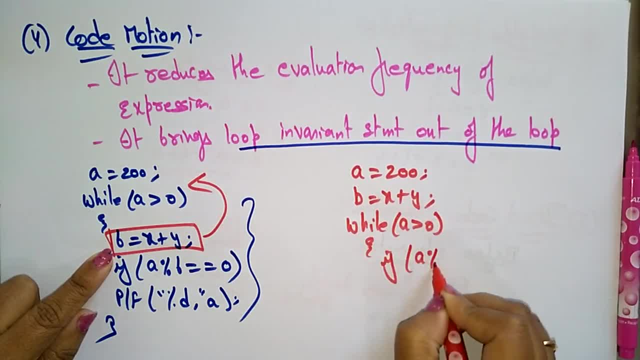 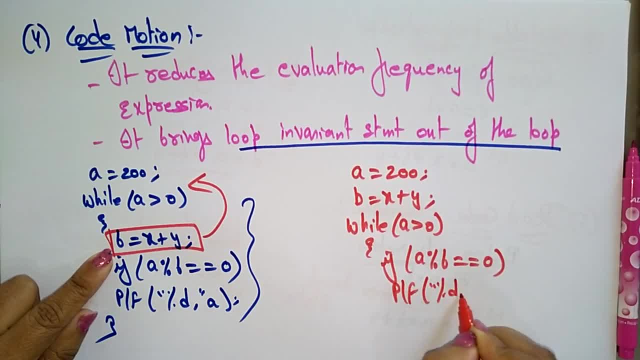 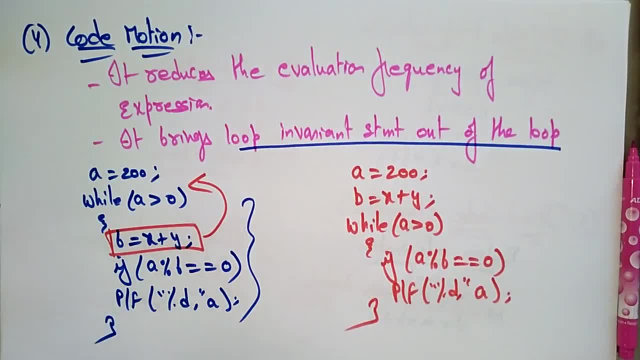 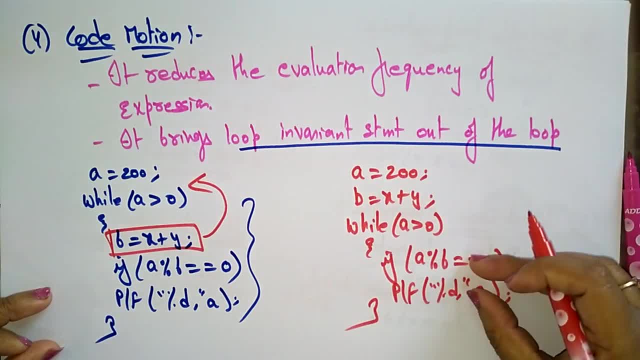 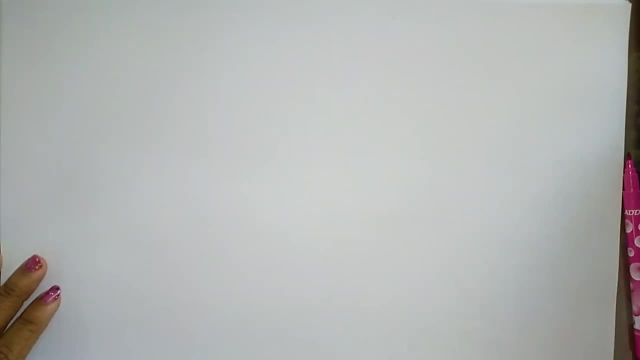 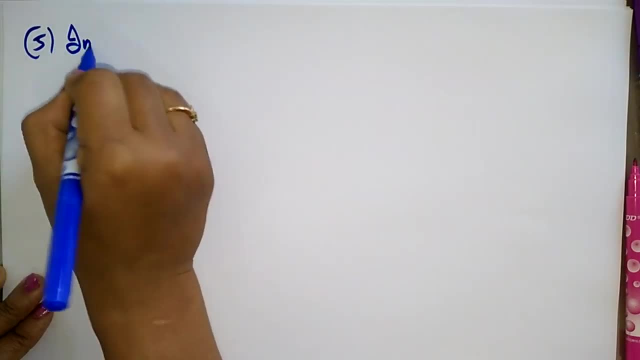 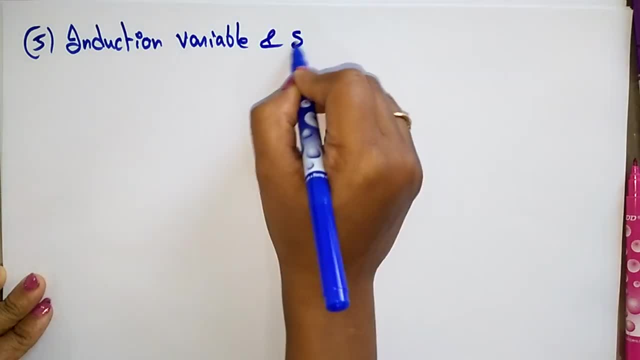 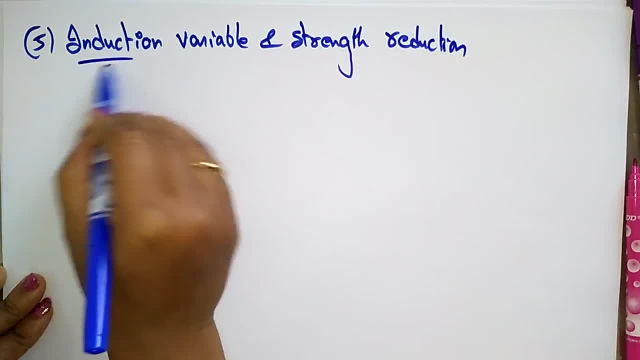 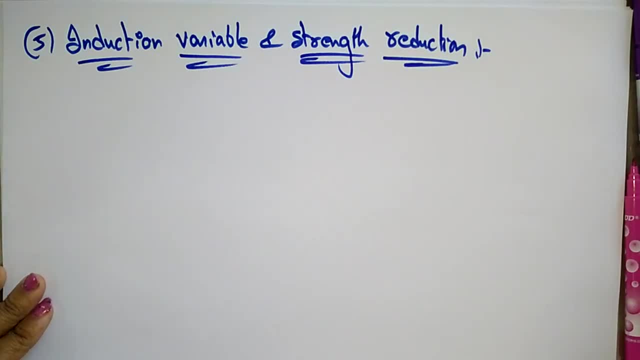 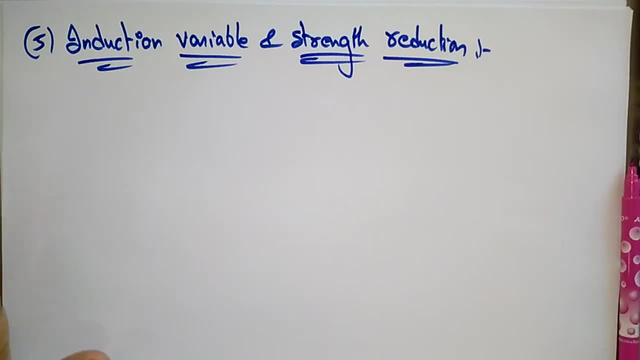 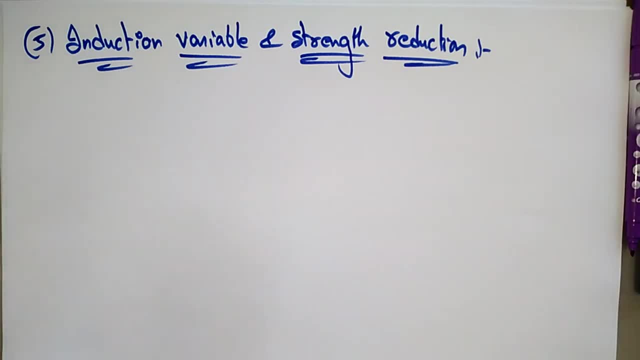 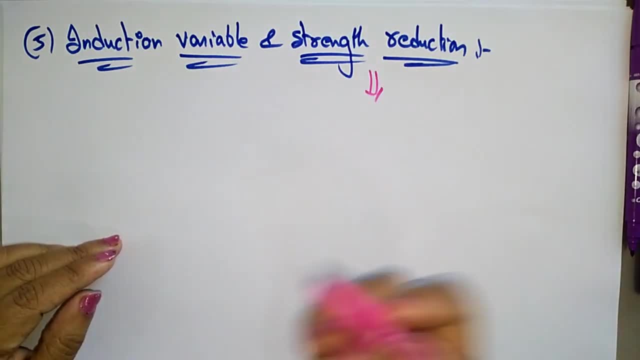 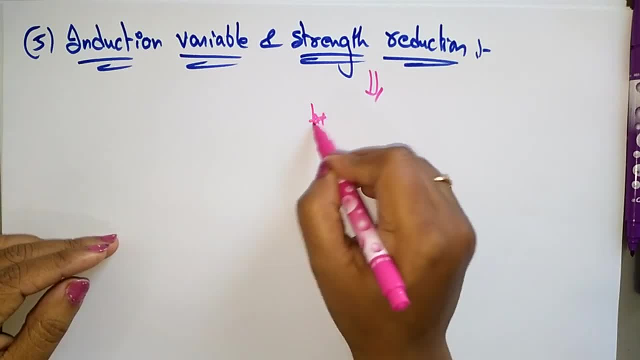 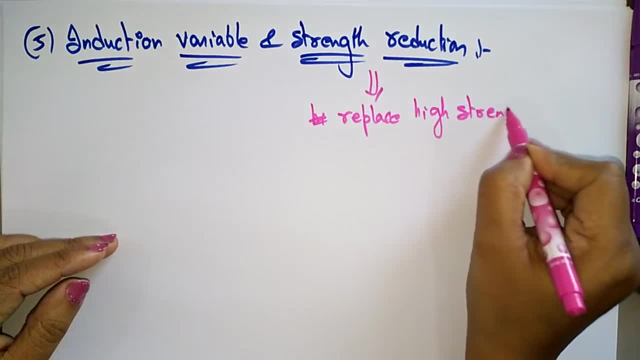 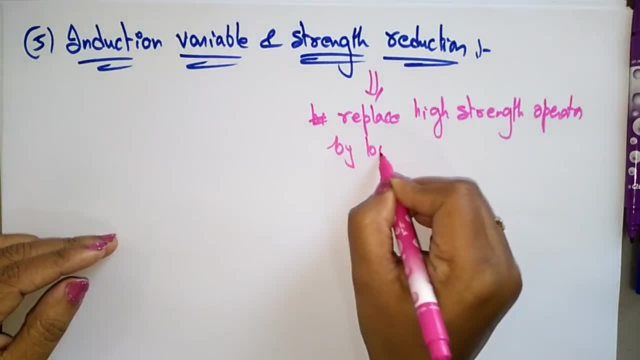 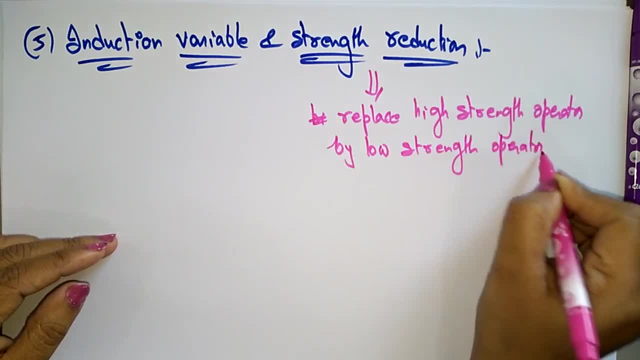 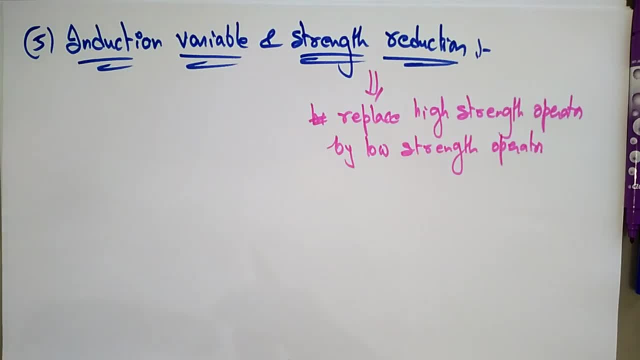 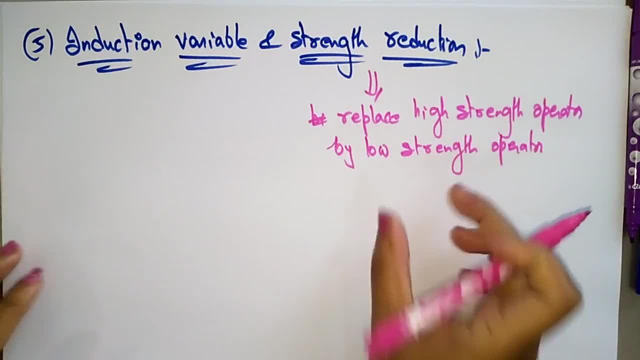 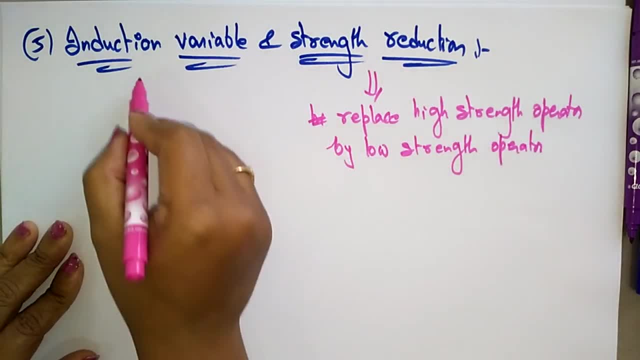 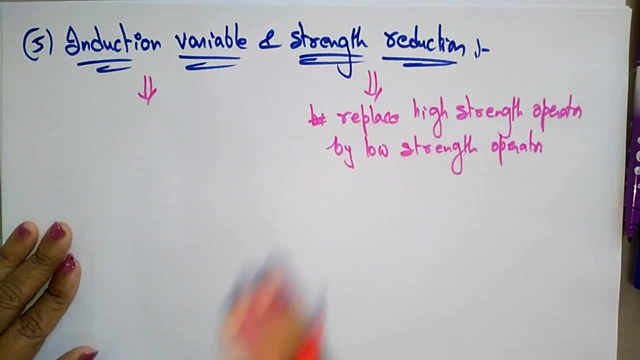 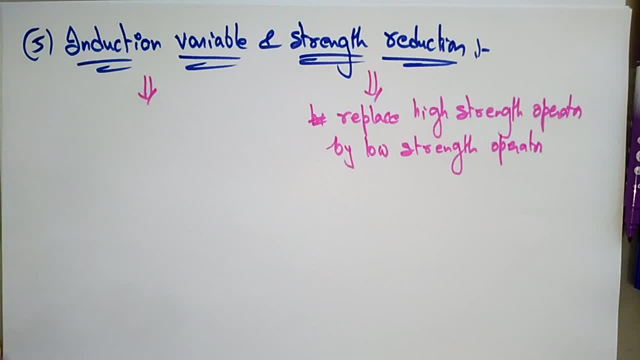 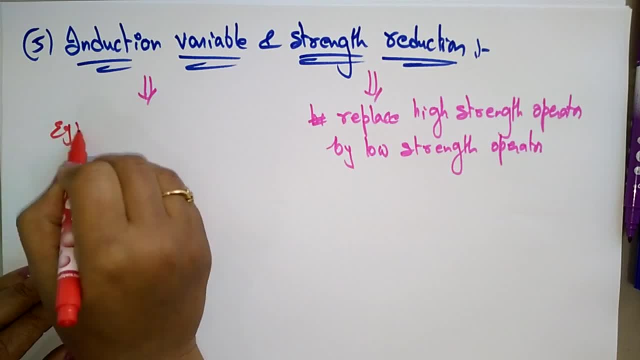 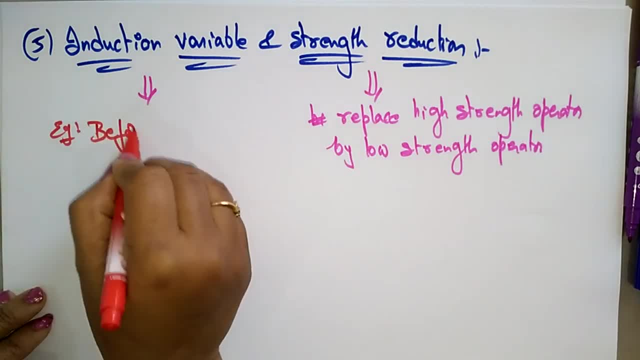 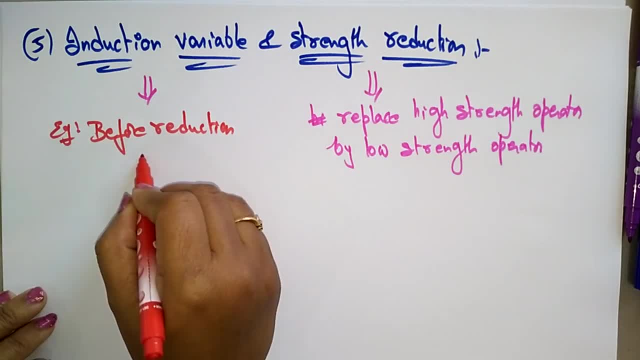 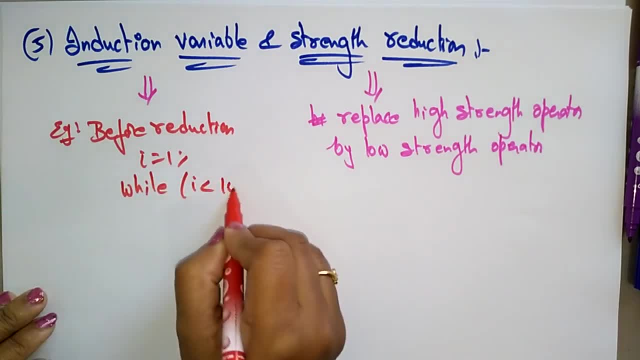 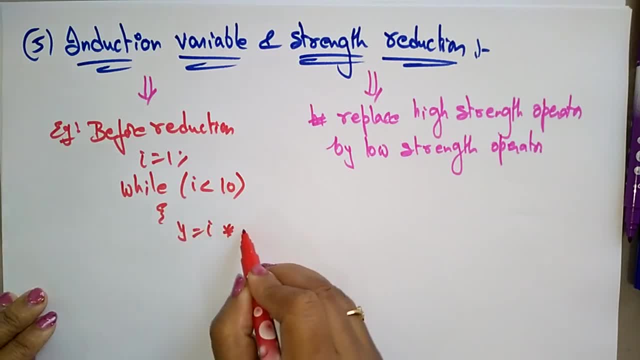 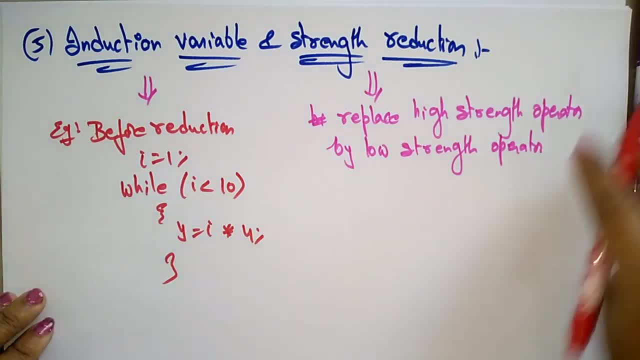 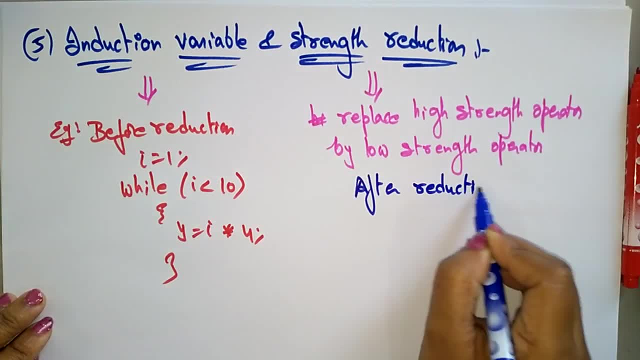 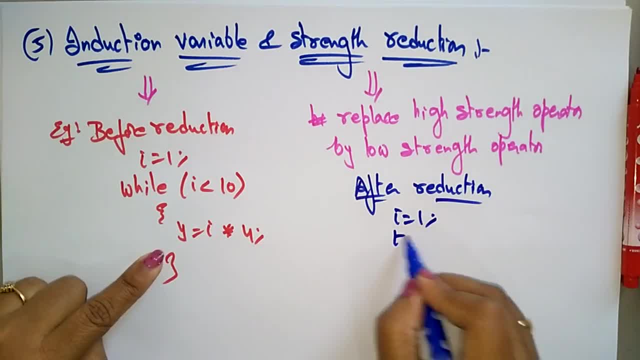 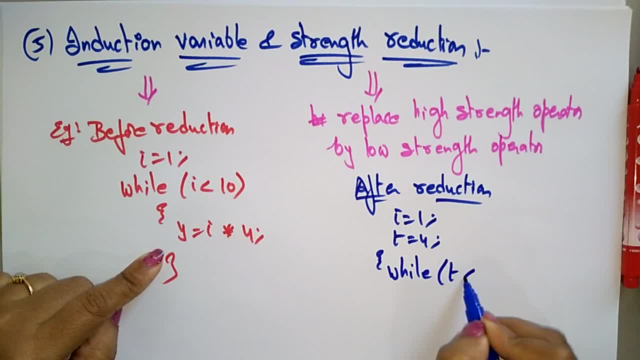 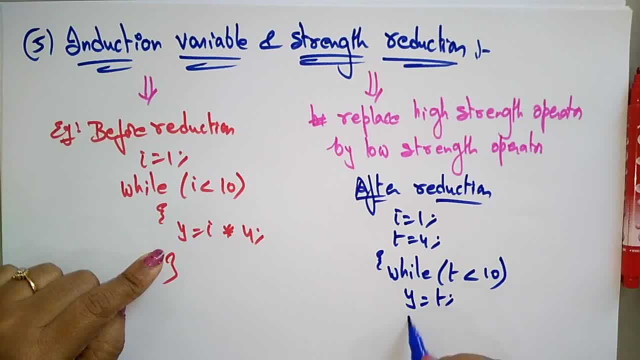 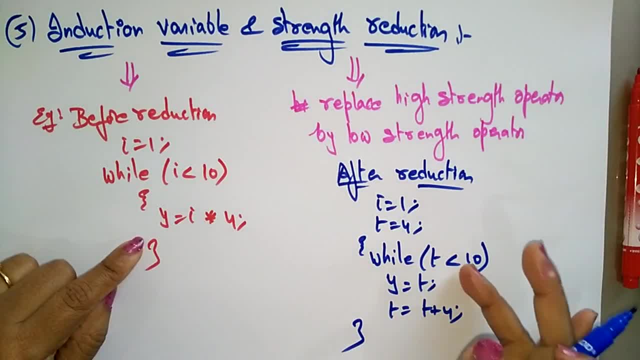 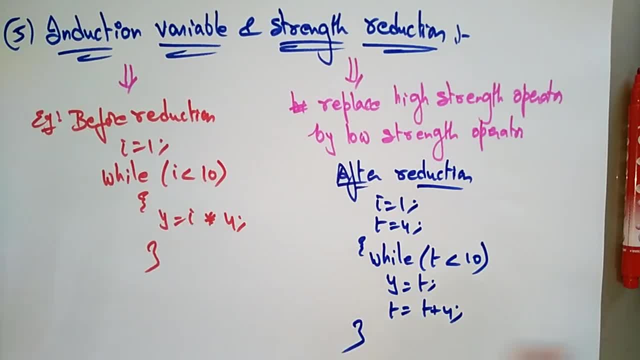 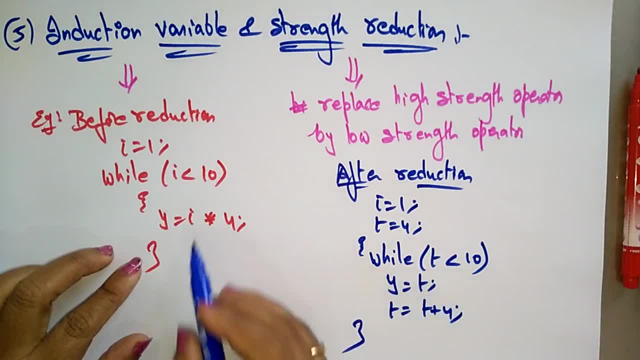 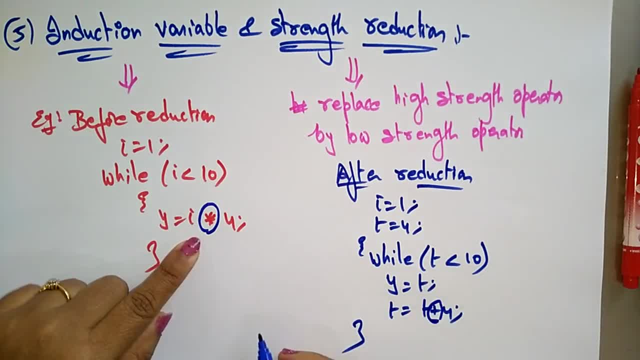 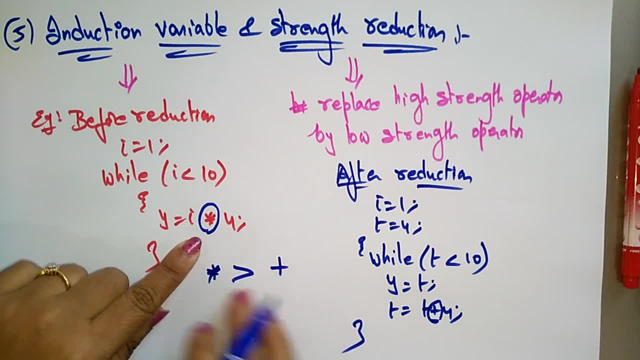 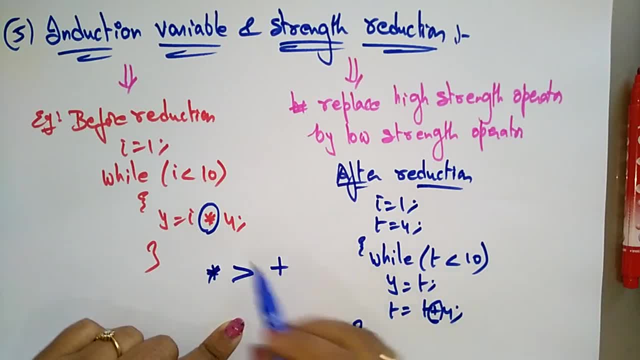 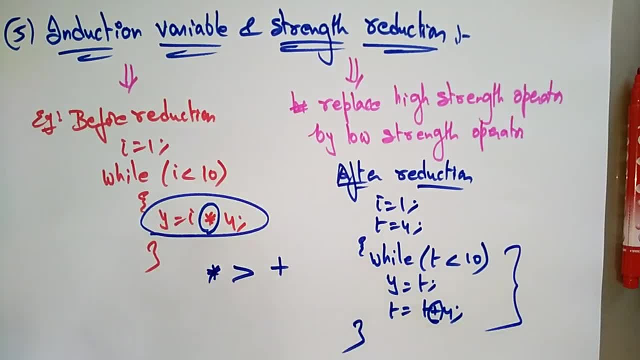 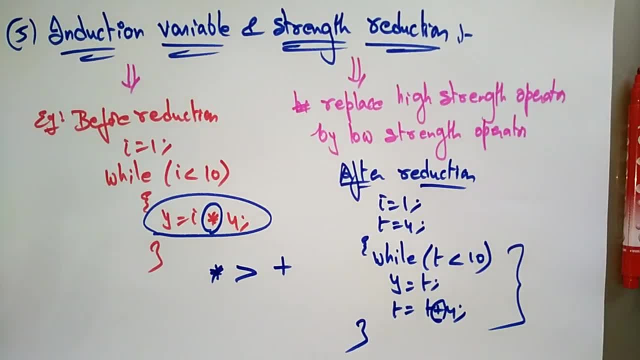 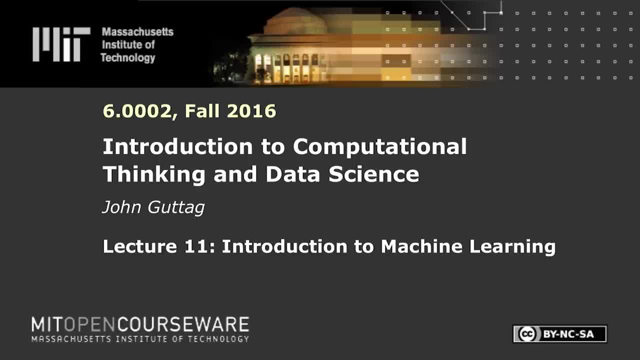 The following content is provided under a Creative Commons license. Your support will help MIT OpenCourseWare continue to offer high quality educational resources for free. To make a donation or to view additional materials from hundreds of MIT courses, visit MIT OpenCourseWare at ocwmitedu. 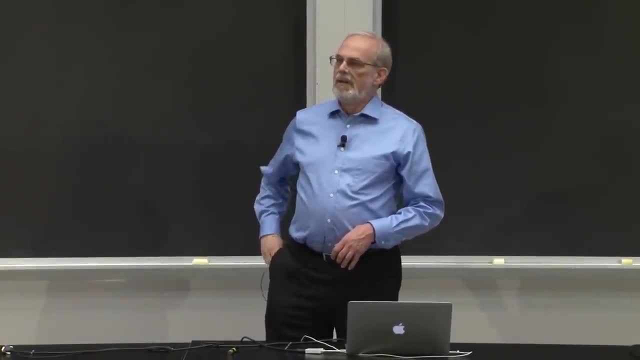 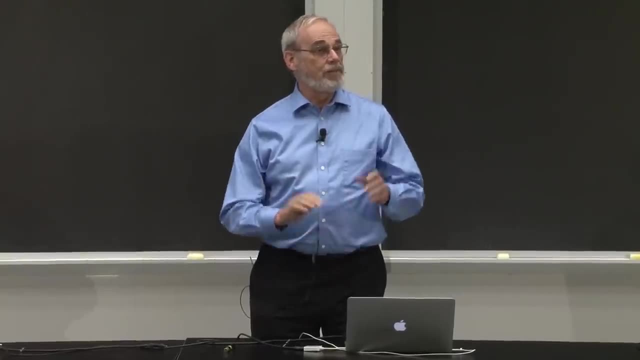 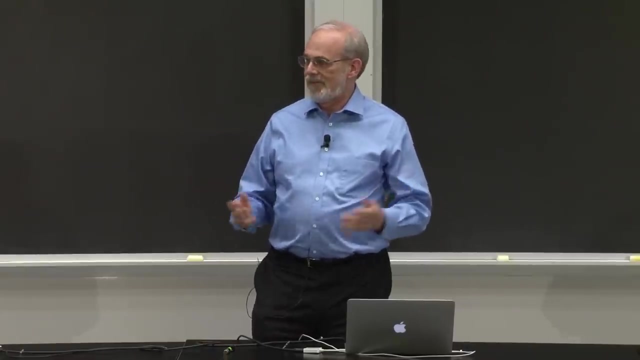 OK, welcome back. You know it's that time of term when we're all kind of doing this, So let me see if I can get a few smiles by simply noting to you that two weeks from today is the last class. Should be worth at least a little bit of a smile, right? 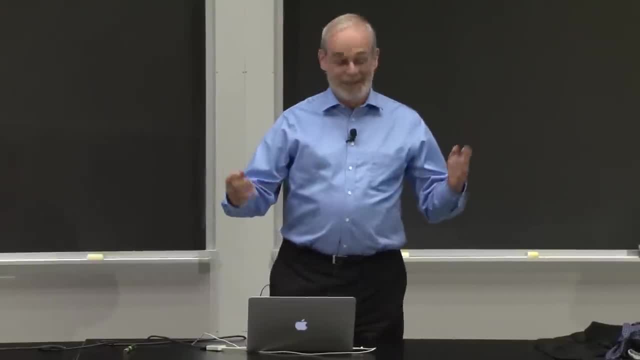 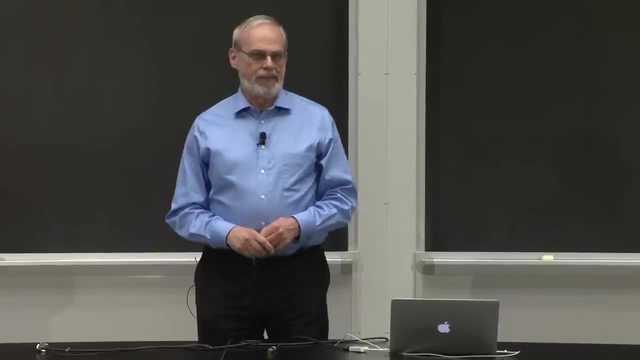 Professor Guttag is smiling. He likes that idea. You're almost there. What are we doing for the last couple of lectures? We're talking about linear regression And I just want to remind you this was the idea of. I have some experimental data. 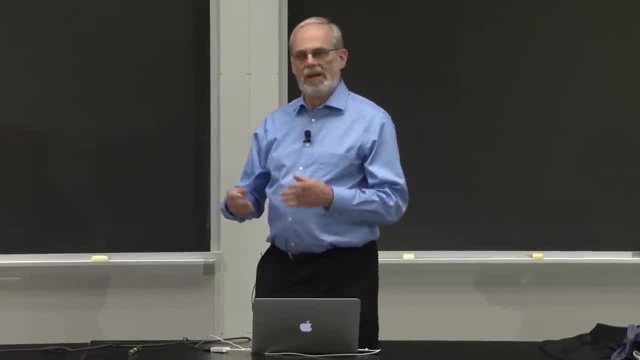 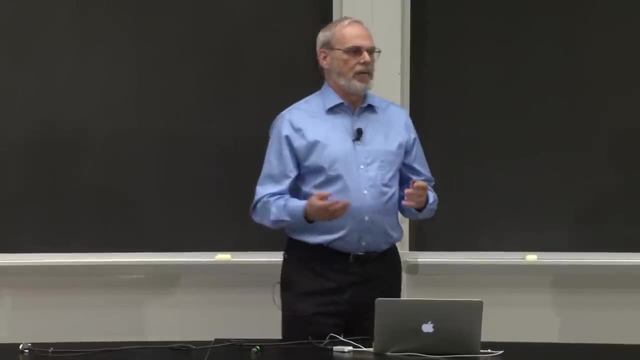 case of a spring where I put different weights on- I measure displacements And regression- was giving us a way of deducing a model to fit that data And in some cases it was easy. We knew, for example, it was going to be a linear model. 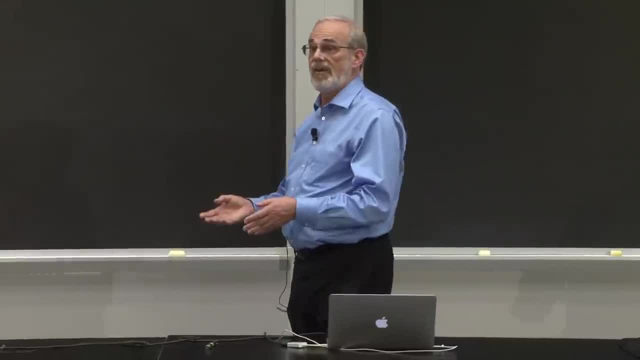 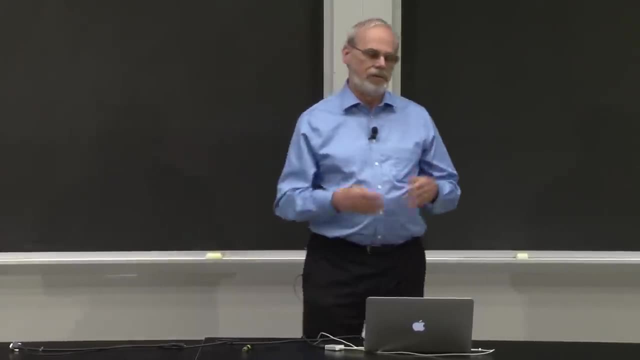 We found the best line that would fit that data. In some cases we said we could use validation to actually let us explore, to find the best model that would fit it, whether it's a linear, a cubic, sorry- a linear, a quadratic, a cubic, some.